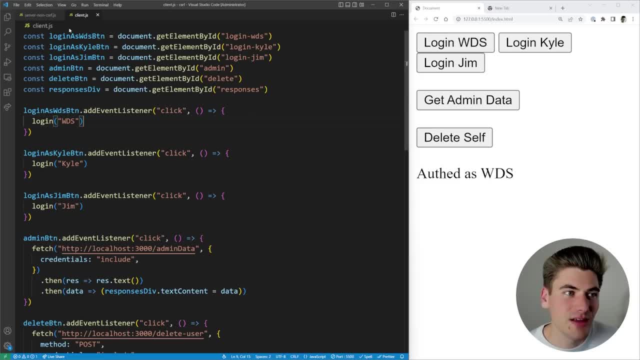 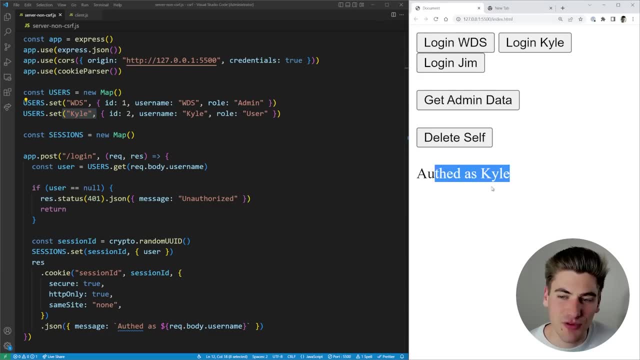 walk you through really quickly. We have three buttons on our page for logging in and on our back end we have users for WDS and for Kyle. So when I click login WDS, I'm off as WDS, Same thing for Kyle, and if I try to log in as Jim, I'm unauthorized because there is no Jim user And 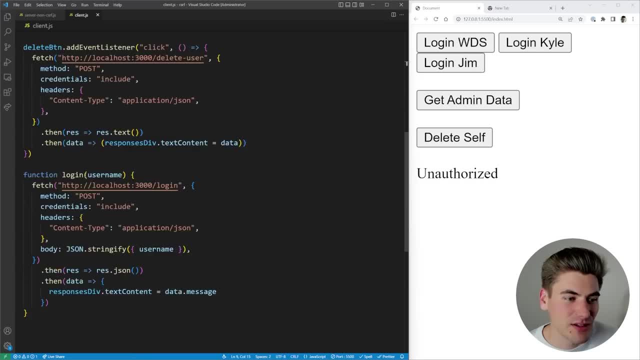 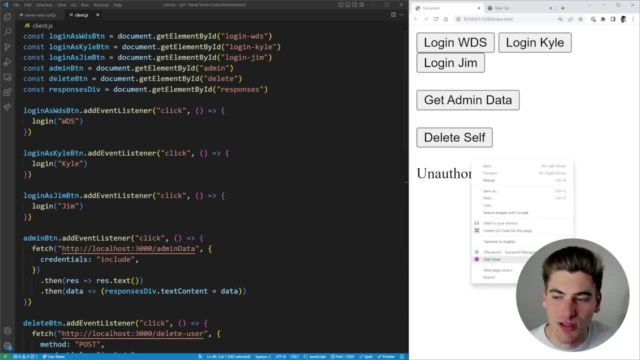 all these functions do is they just make a request to my API that is doing that, logging in right here, just showing that I'm logged in as that user And the important thing is it's sending down a cookie with my session. So if I just inspect my page right here and I go over to the network tab, 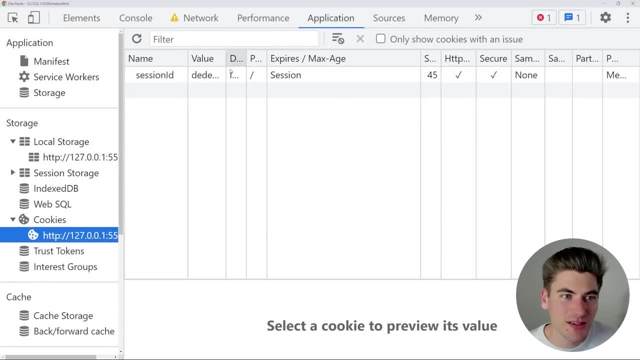 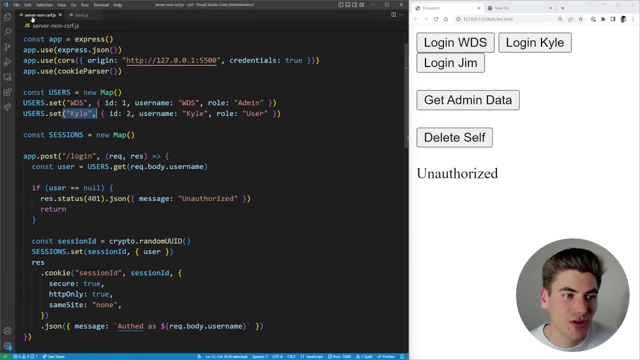 or, I'm sorry, not the network tab, the application tab, and I look at my cookies. you can see we have a cookie for our session ID and it has a long value for my session ID for that current user And in that session on my server I'm saving my user information. So whenever I log in 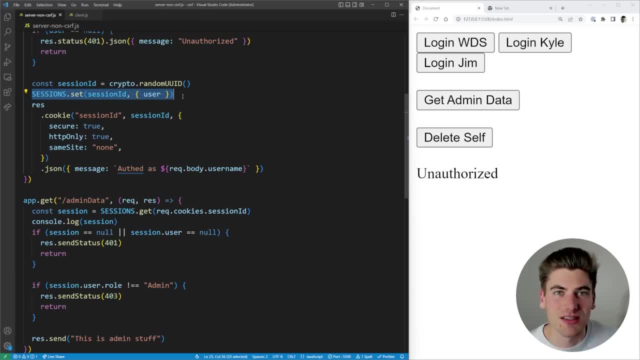 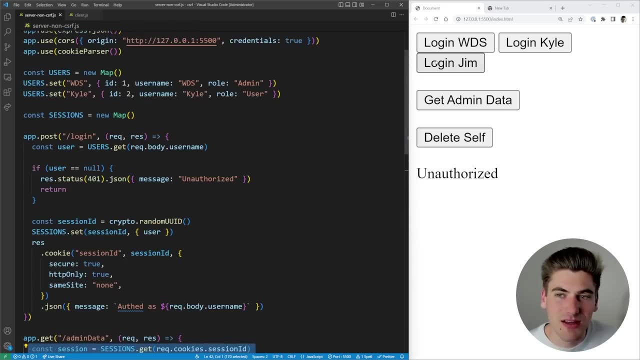 you can see here I'm saving a session that links my user and that session ID. That way, every time I make a request, I send along that session ID and now I can access that user, For example, if I try to get the admin data. So if I log in as WDS and I click get admin. 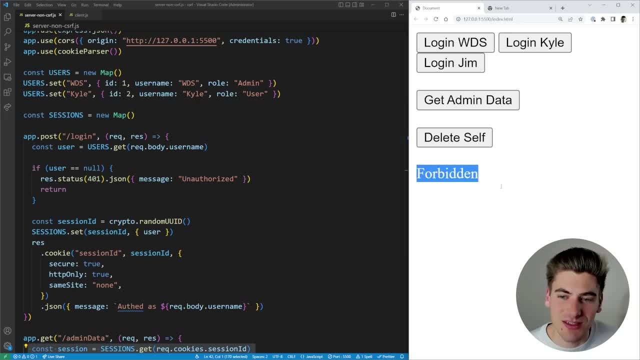 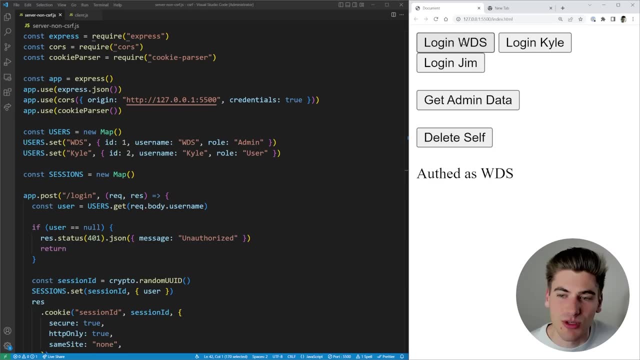 data. you can see it returns, but Kyle is not an admin, So when I try to get the data, you can see we don't have that information being sent to us Now. I also included some other stuff for deleting my account. So if I log in as WDS and I click delete and I try to actually get my admin data, 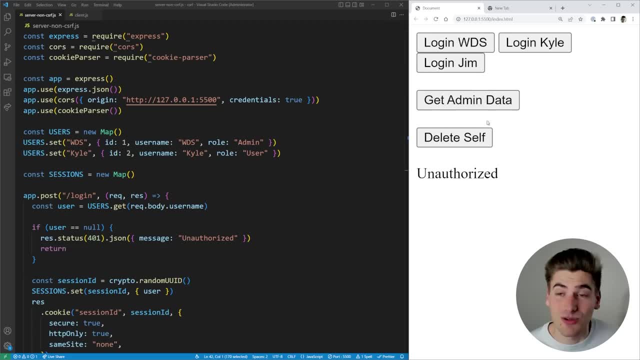 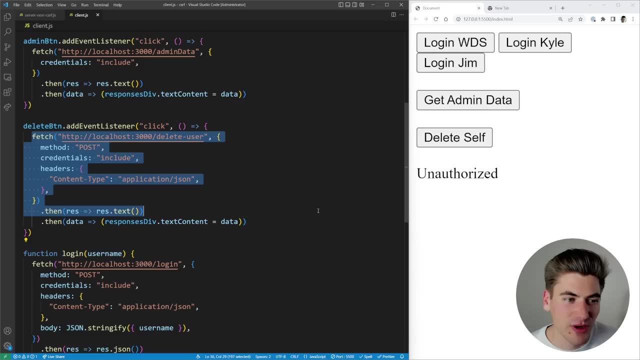 you can see I'm unauthorized. And if I try to log in as WDS, you can see it's not working because there is no account for that user anymore. It's been completely deleted. Now, if we go over to our client, you can see that, in order to make this work, we're just doing a fetch request. 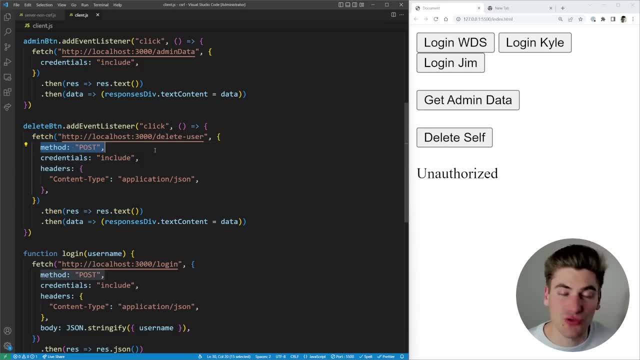 post method request here And that's all that's happening right here. Pretty straightforward stuff. Generally, you'd probably do a delete here if you're doing a delete, But in our case we're using a post because it shows some of the vulnerabilities to cross site request forgery. 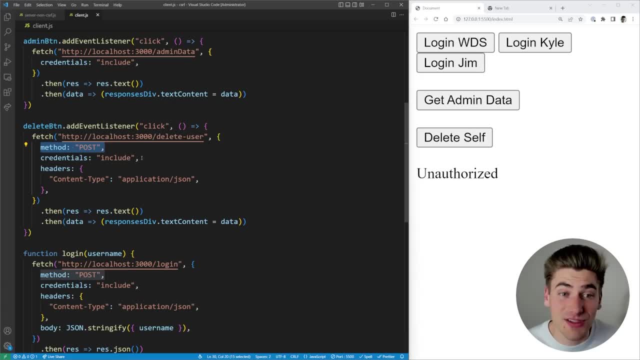 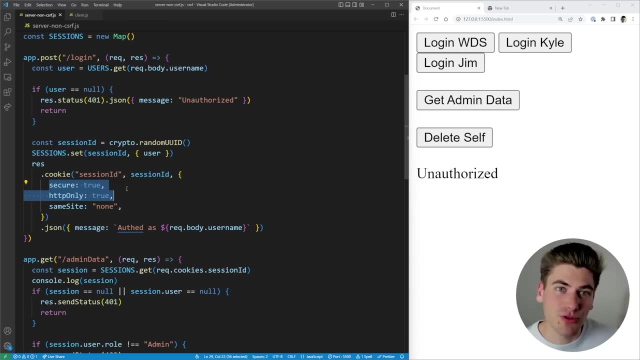 So that's how this all works. How exactly is this vulnerable? Because you may think this is super secure, because when we're saving our cookies, you're noticing we're doing secure and HTTP only. That means that the cookie is never exposed to JavaScript, so no one can steal that session ID. 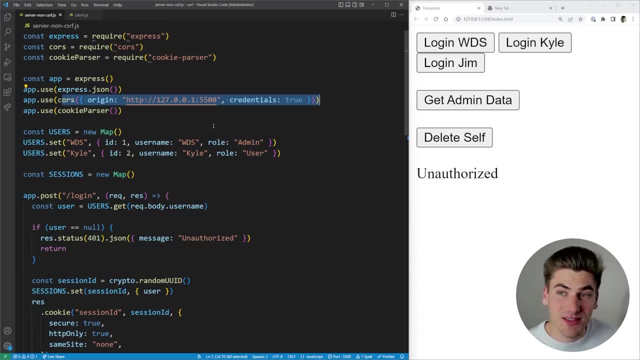 That's great. We also have core setup so it only accepts requests coming from our particular URL. again, That's super great. We can't make requests from some other URL, but we actually can. Cores does not prevent people from submitting forms from other URLs, So what I also have is another. 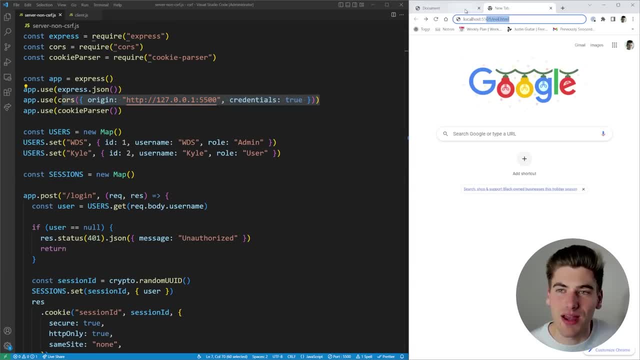 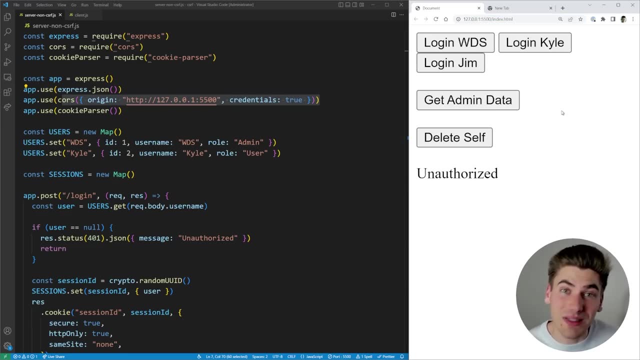 page over here: localhost 5501- evilhtml. It's a completely different URL. I know they're both on localhost, but this is running on a different port And according to cores those are two completely different sites. Normally it would block me if I tried to make a request from that. 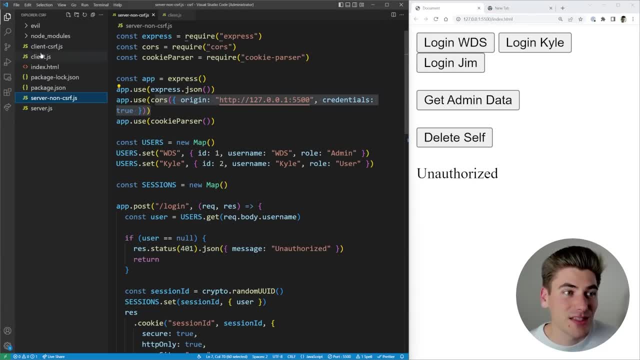 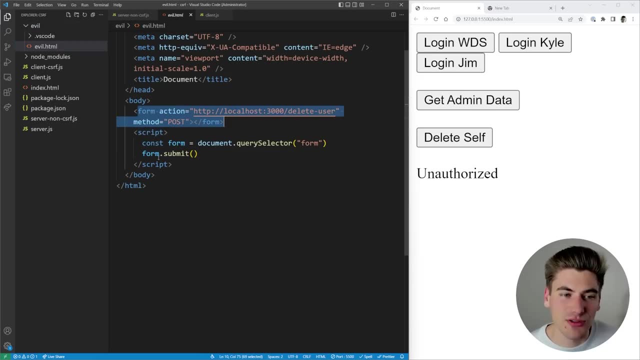 5501 to my normal 5500.. And in this all I'm doing really simply, is I'm making a post action on a form that is going to that delete user, And you can see that this is happening automatically as soon as I go to the page. I don't even need to. 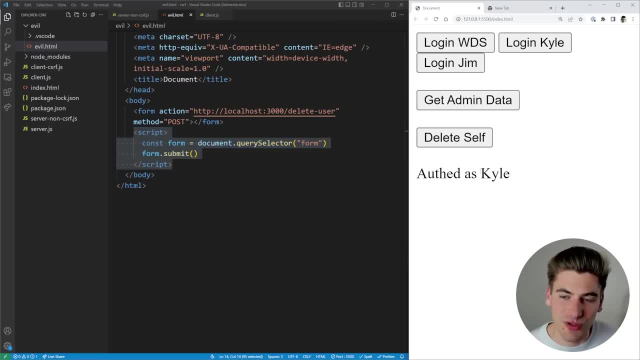 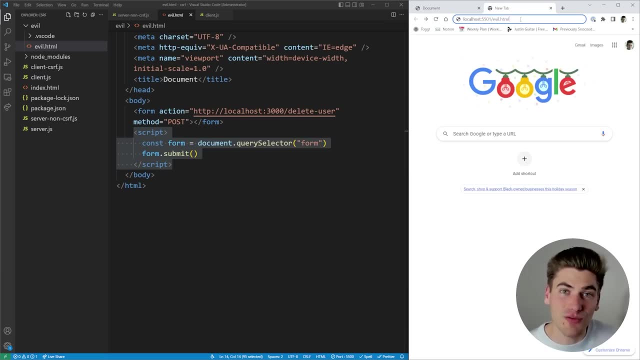 click any buttons at all. So let me real quickly log in as Kyle. You can see I'm authenticated as Kyle. That's super great. Everything is working as we would expect. Now all I need to do is just go to this page. It's on a completely different URL And if I go to this page, you can see it. 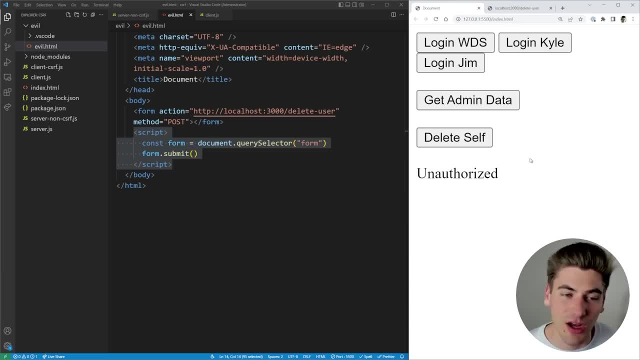 has deleted that Kyle user And if I come in here, try to log in, you can see it's now unauthorized because that Kyle user has been deleted. Now I'm probably wondering how exactly is this possible if you have core set up and all these? 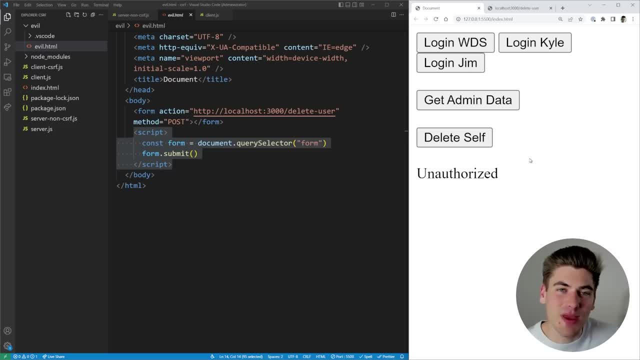 other precautions, And the reason for this is every single time that you make a request to a server, the cookies are sent along automatically. So I was logged in as Kyle on this page, So my cookie for that Kyle session was already saved in the cookies And then, when I made a request to 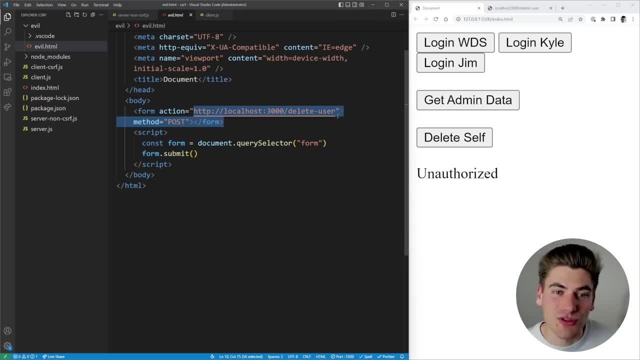 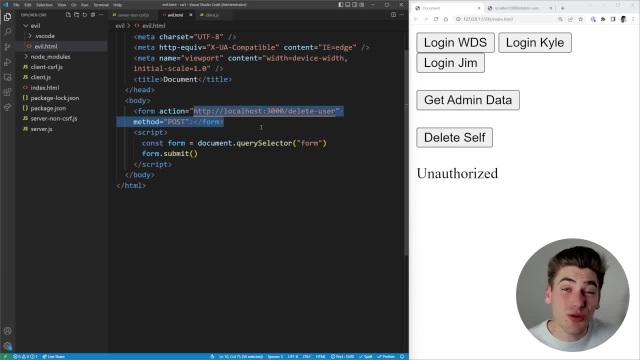 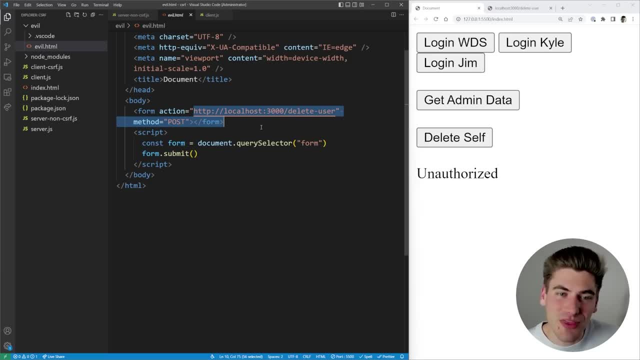 doesn't actually prevent a lot of things. It's not really a great security method per se because it doesn't prevent like servers from communicating with other servers. Now that particular use case of servers calling other servers isn't important in this case, because your cookies aren't saved. 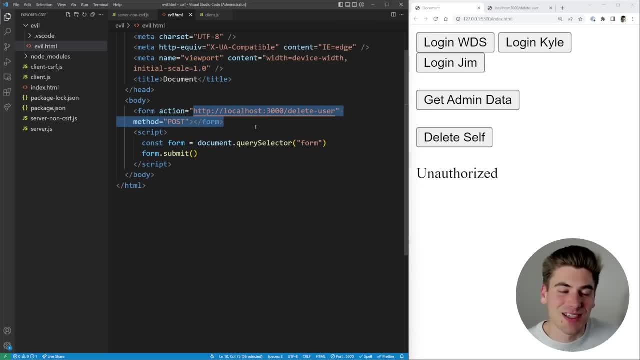 on the server. But it is just something to know that cores is not really a security measure. It's more just something there to try to help with certain things, But it shouldn't be seen as like an all be all security measure. So we're getting around our course and we're able to send requests. 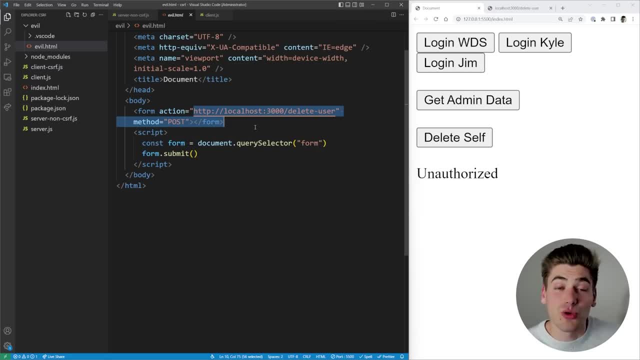 using the cookies of that user that are saved in the cookies. So in order to make sure that this request problem doesn't happen, we need to have some other type of validation that is not saved in the cookies. That way it's not automatically sent along with our request, And if we look at 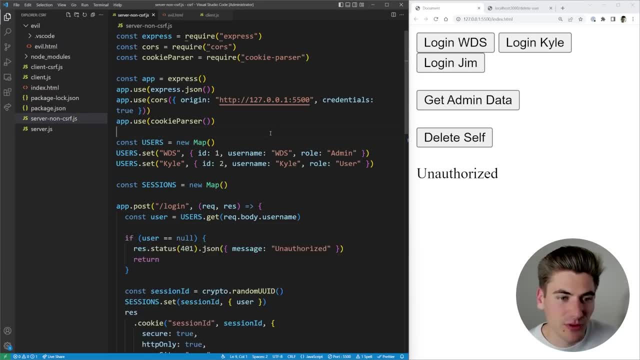 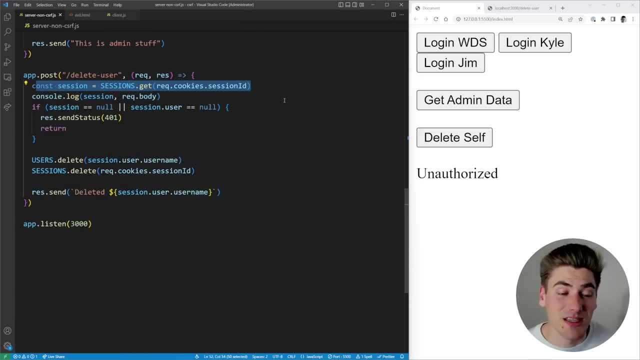 our server here, our non CSFR version. this is the version that is vulnerable. you can see that it's very basic stuff, But essentially in our delete request here all we're doing is we're getting our session And we're checking to see if we have a user, And if we do have a user, then we're. 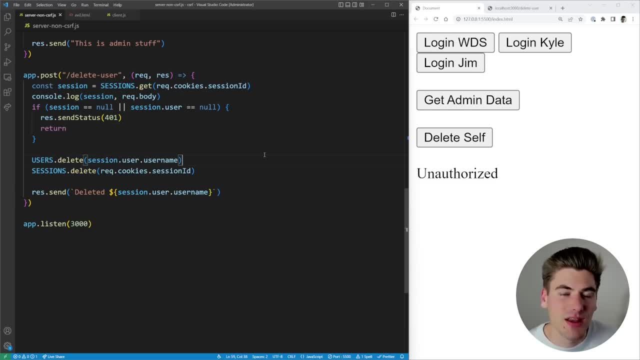 deleting them and we're deleting their session. pretty straightforward stuff. Now let me show you how this CSR of our version works, where we have some other piece of validation. Let me open that up real quick. we have our normal server here. I'm actually going. 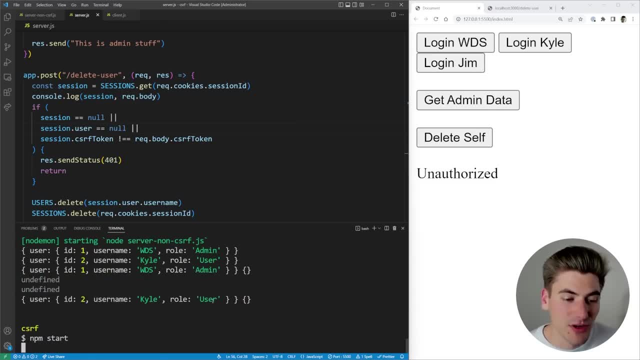 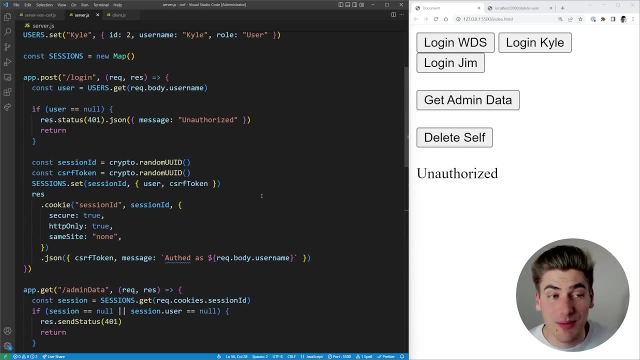 to run that instead of our other server. So I'm just going to start this up. this is going to be for our correct version of our application. Here we go. So what this correct version does is when we log in, we have a additional step. that's happening is we're creating this random token. 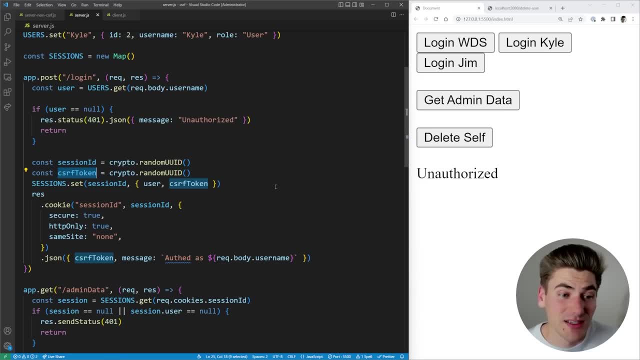 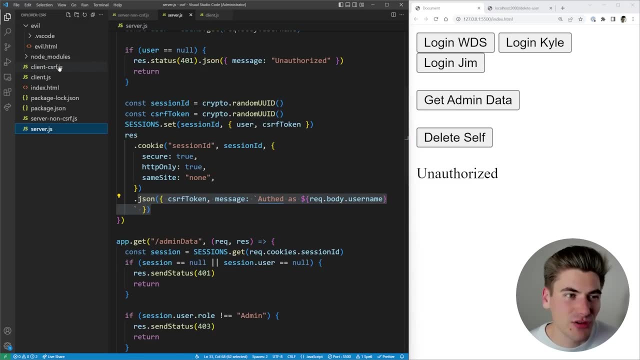 doesn't matter what it is. it's just a random string of values which is used for authentication purposes And we're making sure we send that random value down to our user on the client Then if we make sure that we use the correct client. so this right here is all the. 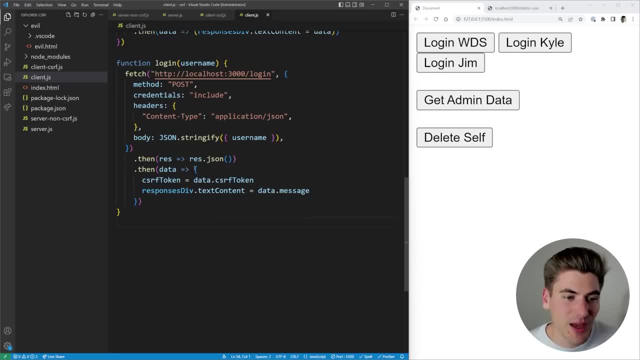 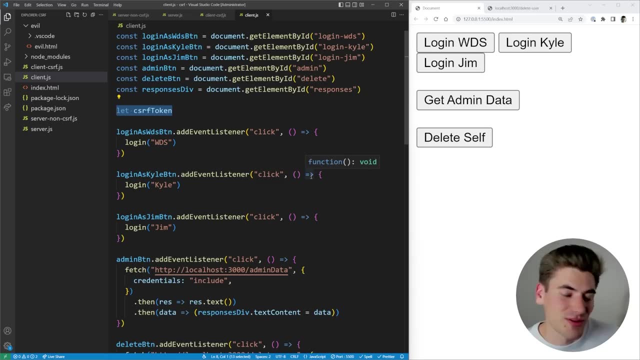 correct code. I'm just going to paste this in. it's almost identical. you can see what happens when we log in. what we're doing is we're just saving that CSFR token instead of a variable here, So just being saved locally in our JavaScript. there's no way any other site could. 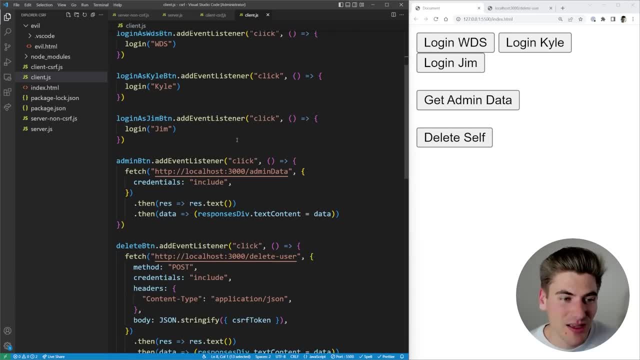 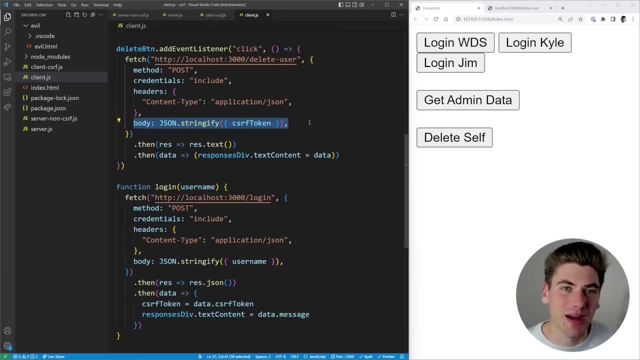 access. this is not saved anywhere else. And then what we're doing is anytime we send along a request- for example, we want to delete our user- we make sure we send along that CSRF token inside of the body. Then if we go check our server real quick we can actually see inside of the body there's. 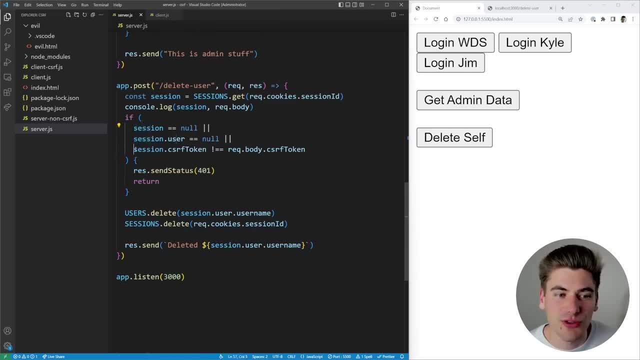 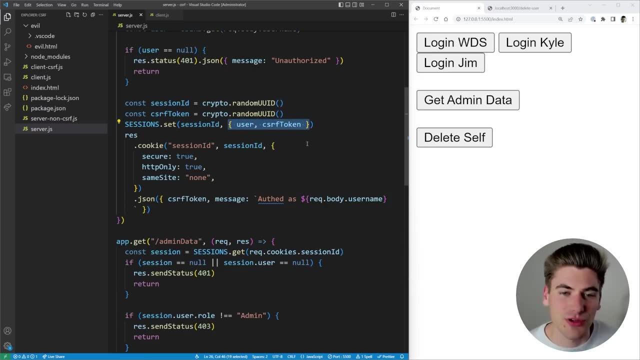 no way that we're going to be able to access that user. So if we go inside that delete function, instead of just checking our session, we're also checking to make sure the CSFR token is matching, And you'll notice that when we create our session we link that together with our user and our token. 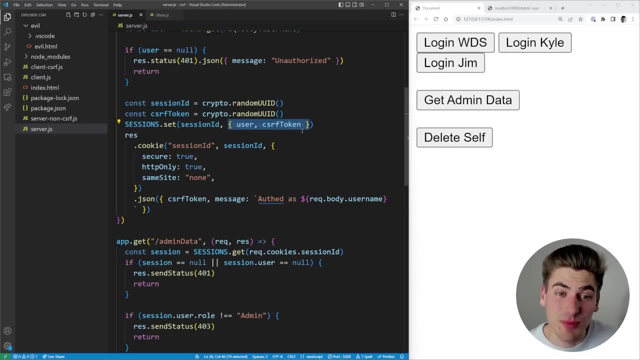 So every single session has a token and it's going to have a user and we need to make sure not only does our session ID match, but also our CSFR F token matches. So if we want to see if this is working, let's just refresh everything on our page. I'm going to log in as Kyle get my data. that worked. 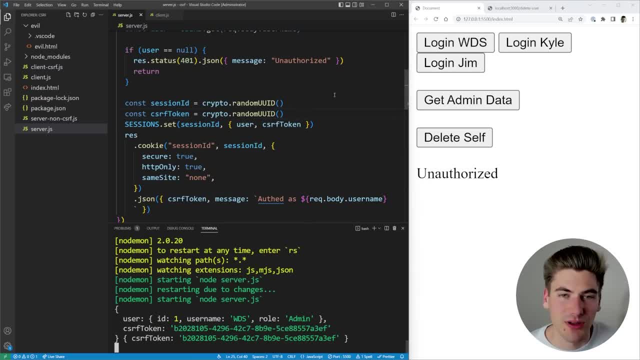 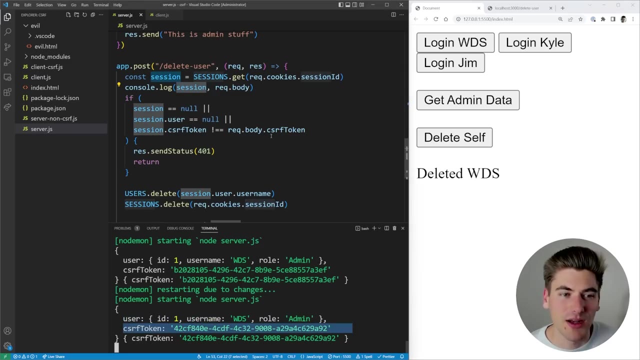 fine, delete and log in. everything you can see is working just fine And when I click delete, you can see it's passing along some information. If we look at what we're logging out, we're logging out our session, which is the first object, which is our user and our token, and we're logging out the body. 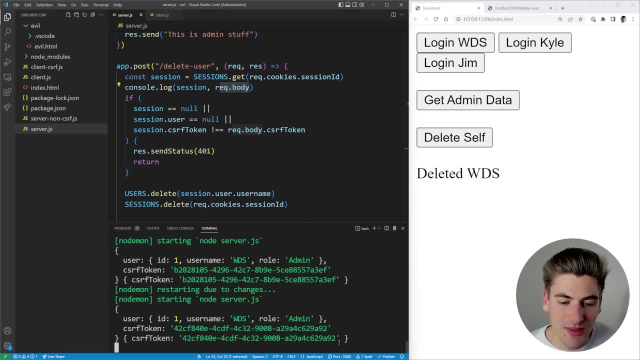 that's being passed up, which, in our case, is also just this token, And these two tokens are exactly the same, they match, which is why our request is going through just fine, But let's see what happens when we go over to that evil. 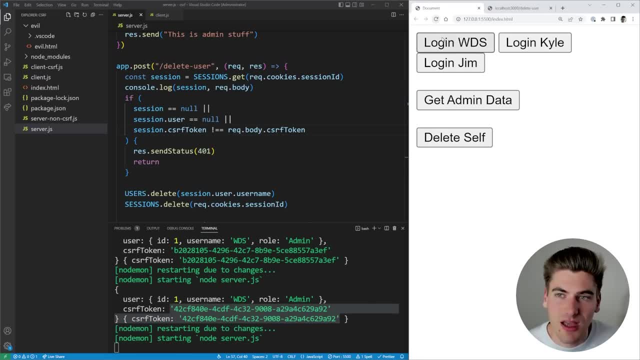 version of our page. So let me just make sure I refresh everything again. I'm going to log in as WDS And then what I want to do is I want to go to that URL, which is 5501- evilhtml, And when I hit enter, you're going to notice we get an unauthorized error. And if we look at what's, 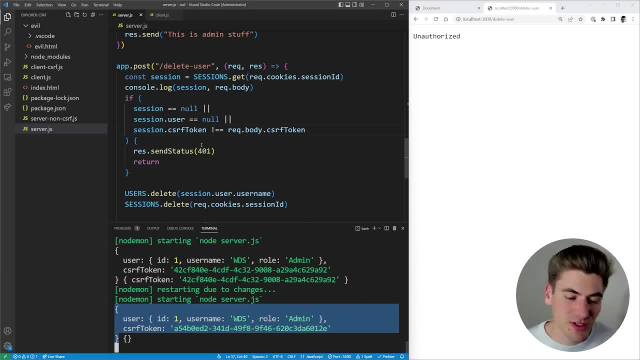 being printed on our console. you can see the session has properly been caught. we're saying: hey, we know that this is the WDS user, based on their session ID, but we didn't pass a CSRF token over to our API. So this check right here where it checks to see if the token in our session is. 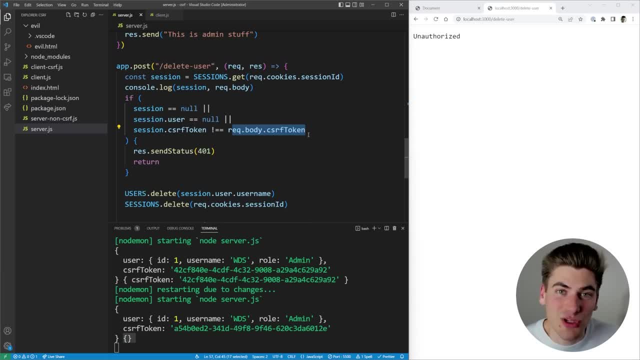 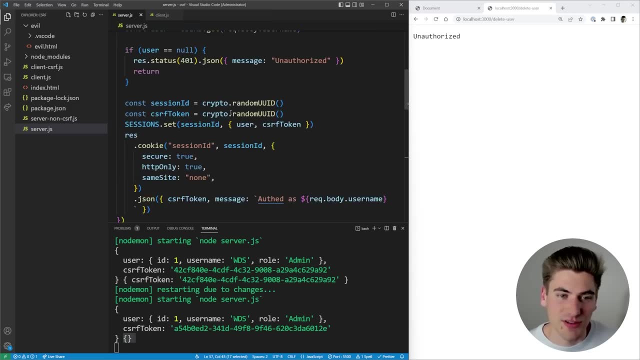 the same as the token in our body is obviously going to fail. there is no token in our body, And this is the key to preventing these different vulnerabilities. Essentially, all you're doing is creating a random string of characters. In our case, 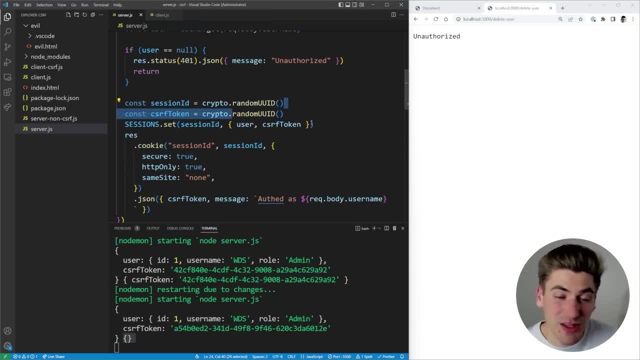 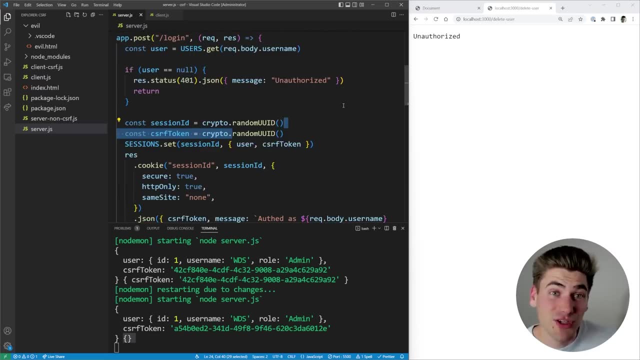 it's just a random UUID. it doesn't matter what it is, it just has to be random, completely random. you're giving that to the user And you're saying, whenever you make a request, send us this random information And as long as that random information matches the random information we gave you when. 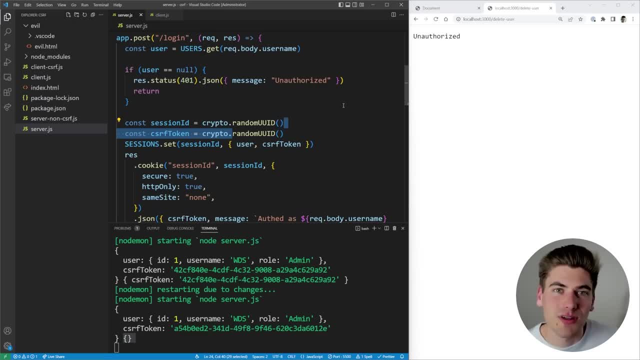 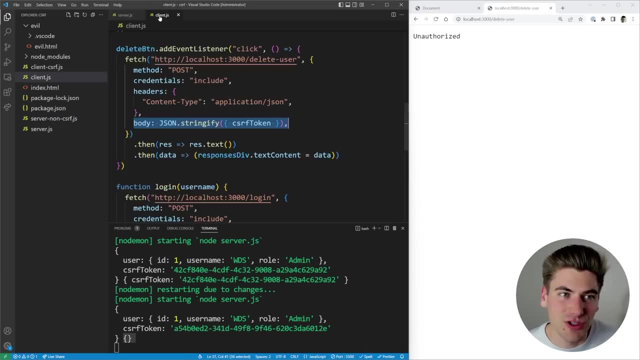 you actually logged in, then you're fine, good to go, doesn't matter, everything works. But if a site is trying to steal your information and pretend to be you, they're not going to have that random information Because, as you can see, we didn't store it anywhere, It's just stored. 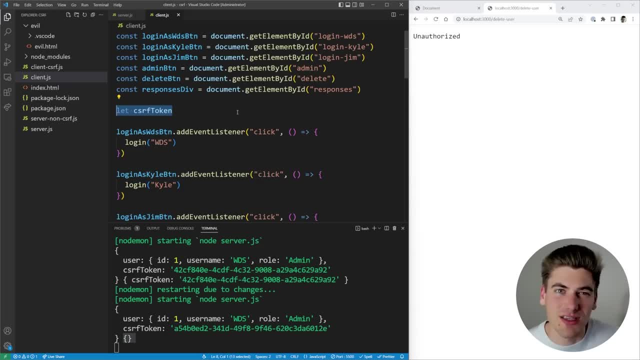 locally inside of JavaScript. it's not stored in local storage, it's not stored in cookies, And that's the key. Generally, you don't want to store this anywhere. you just have it locally on your JavaScript or locally in your form somewhere like as a hidden element. That's going to be fine. 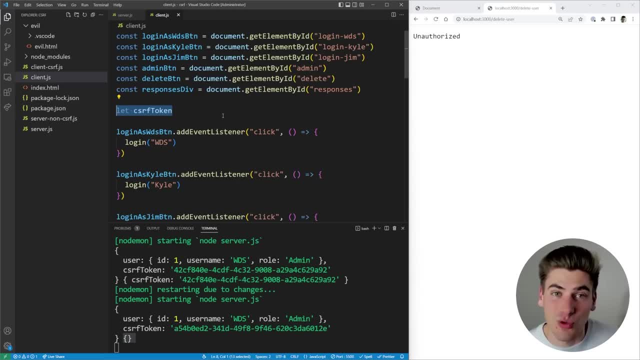 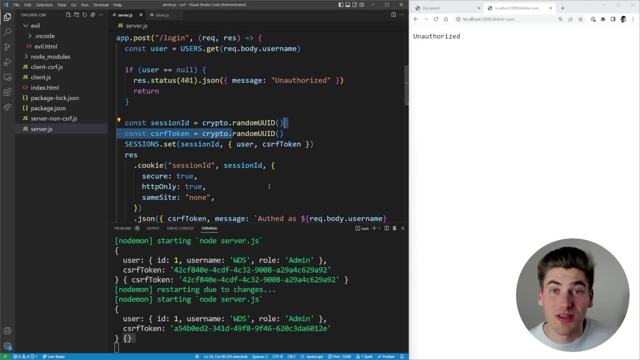 because there's no way this other site has access to that information, because it's not stored anywhere at all, And you just pass that along whenever you make an API request. And that, right, there is what: doubly authenticate you first. you authenticate you are yourself, And then this: